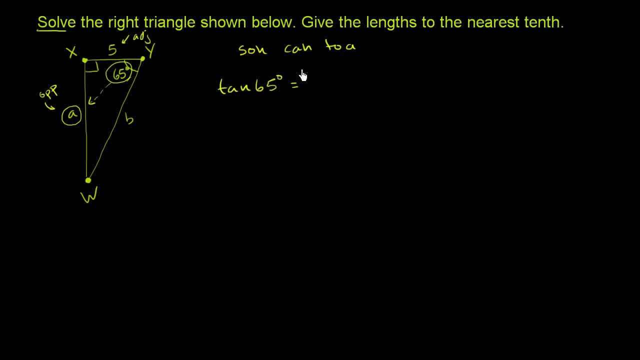 is equal to the length of the opposite side, which we know has length a, over the length of the adjacent side, which they gave us in the diagram, which has length 5.. And you might say: well, how do I figure out a? 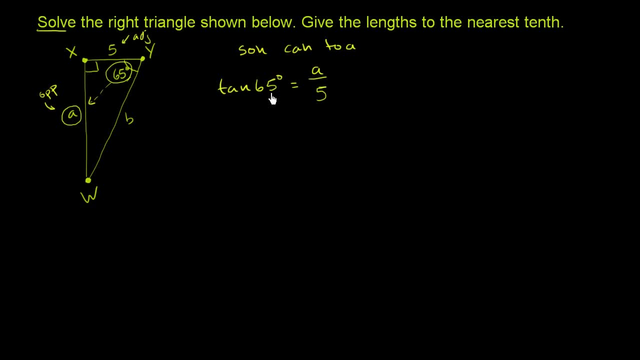 Well, we can use our calculator to evaluate what the tangent of 65 degrees are, and then we can solve for a. And actually, if we just want to get the expression explicitly solving for a, we could just multiply both sides of this equation times 5.. 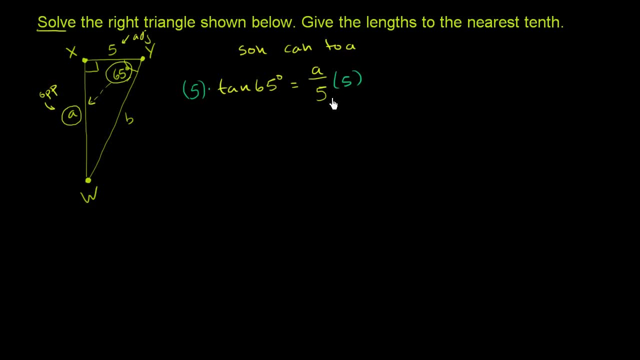 So let's do that 5 times 5.. These cancel out and we are left with: if we flip the equal around, we're left with: a is equal to 5 times the tangent of 65 degrees. So now we can get our calculator. 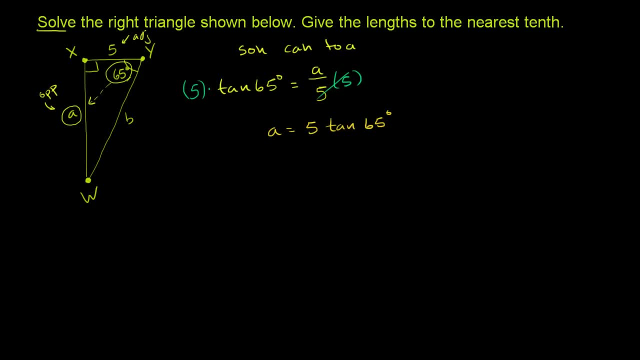 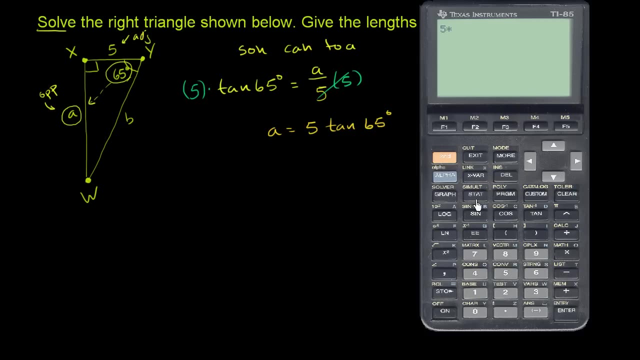 And figure out what this is to the nearest tenth, Get my handy TI-85 out And I have 5 times the tangent. No, I didn't need to press that second right over there, Just the regular tangent of 65 degrees. 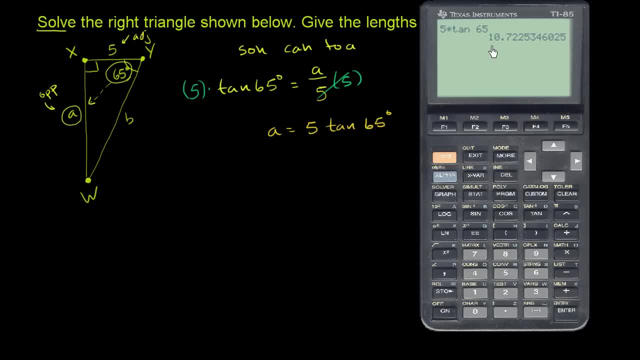 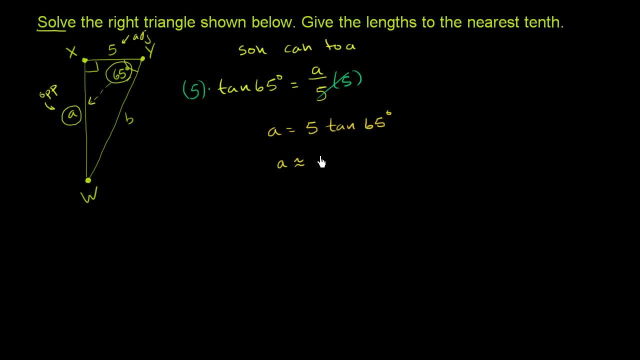 And I get. if I round to the nearest tenth, like they asked me to, I get 10.7.. So this is So. So a is approximately equal to 10.7.. I say approximately because I rounded it down. 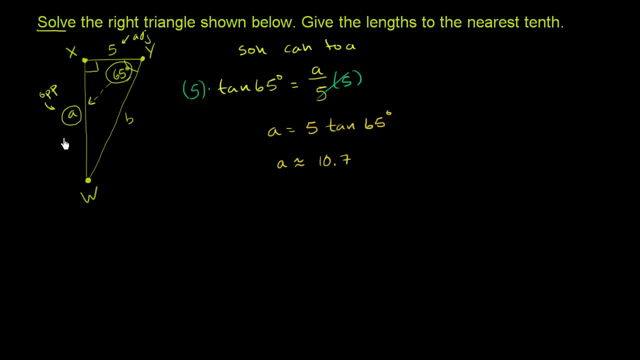 This is not the exact number, But a is equal to 10.7.. So we now know that this has length 10.7, approximately. There's several ways that we can try to tackle b, And I'll let you pick the way you want to. 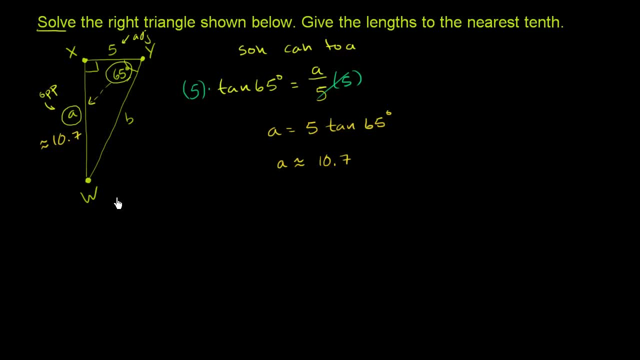 But then I'll just do it the way I would like to. So my next question to you is: what is the length of the side, Side yw, Or what is the value of b? Well, there's several ways to do it. 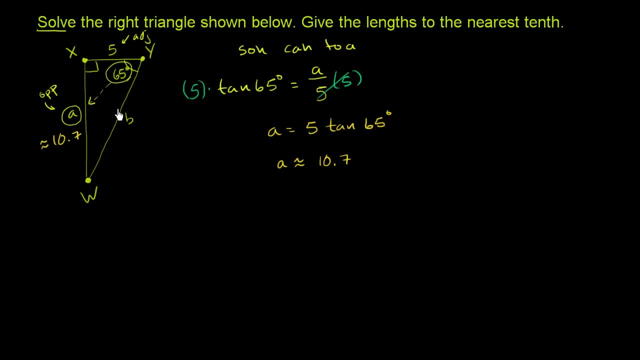 This is a hypotenuse, So we could use trigonometric functions that deal with adjacent over hypotenuse or opposite over hypotenuse, Or we could just use the Pythagorean theorem. We know two sides of a right triangle. We can come up with the third side. 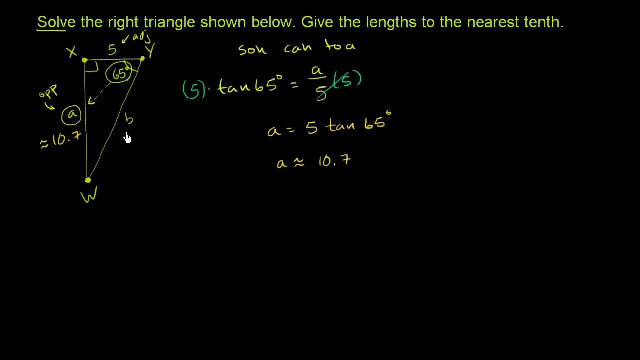 I will go with using trigonometric ratios, since that's what we've been working on a good bit. So this length b, that's the length of the hypotenuse. So this side wy is the hypotenuse, And so what trigonometric ratios? 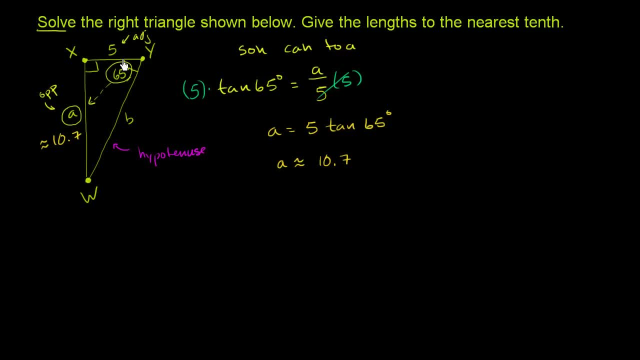 and we can decide what we want to use. We could use opposite in hypotenuse. We could use adjacent in hypotenuse, Since we know that xy is exactly 5, and we don't have to deal with this approximation, let's use that side. 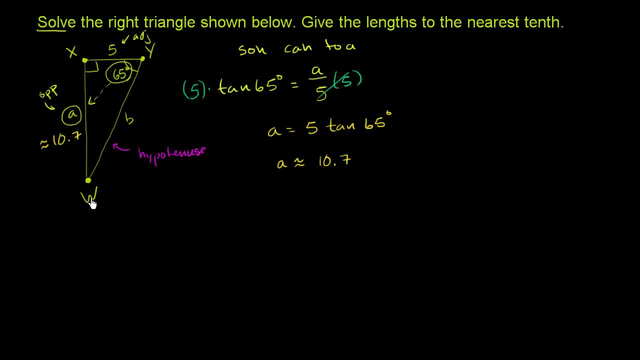 So what trigonometric ratios deal with adjacent and hypotenuse? Well, we see from SOHCAHTOA, cosine deals with No, with adjacent over hypotenuse. So we could say that the cosine of 65 degrees is equal to the length of the adjacent side which. 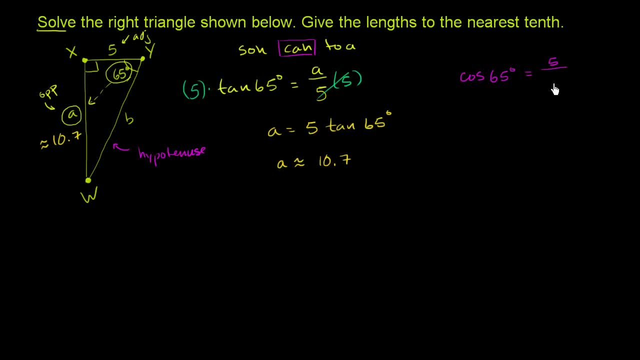 is 5, over the length of the hypotenuse, which has length b, And then we can try to solve for b. You multiply both sides times b, You're left with b. times cosine of 65 degrees is equal to 5.. 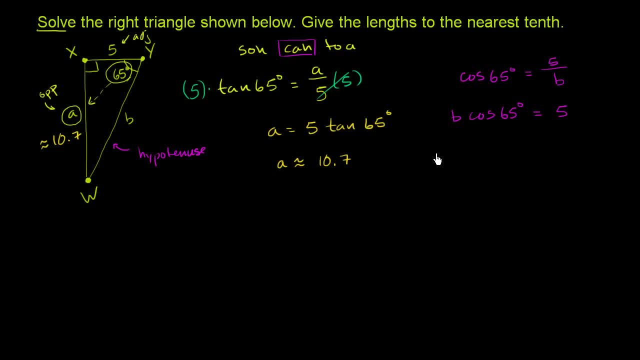 And then to solve for b, you could divide both sides by cosine of 65 degrees. This is just a number here, So we're just dividing. We have to figure it out with our calculator, But this is just going to evaluate to some number. 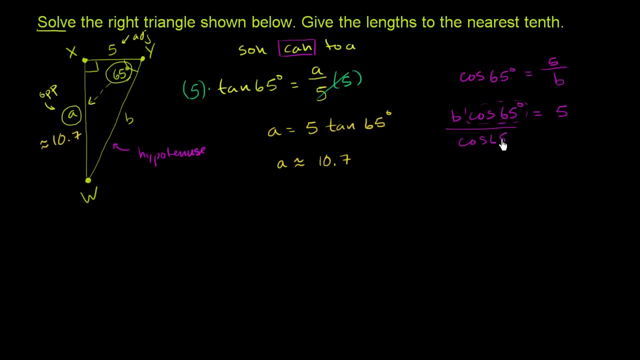 So we can divide both sides by that, by cosine of 65 degrees, And we're left with: b is equal to 5 over the cosine of 65 degrees. So let us now use our calculator to figure out the length of the hypotenuse. 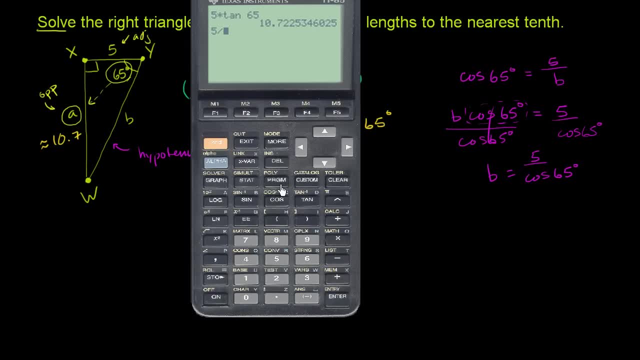 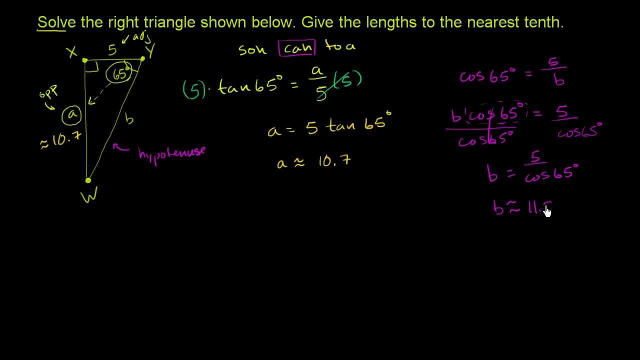 Length of b is 5 divided by cosine of 65 degrees And I get, if I round to the nearest tenth, 11.8.. So b is approximately equal to rounded to the nearest tenth 11.8.. So b is equal to 11.8.. 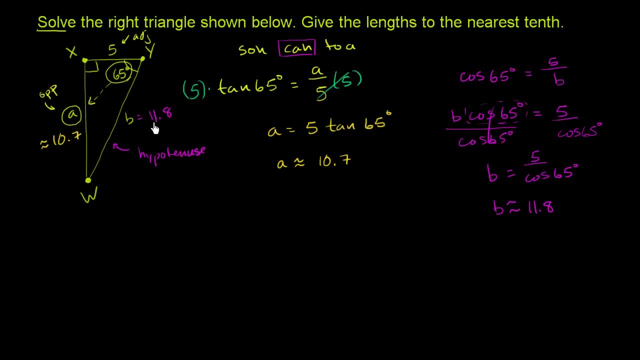 And then we're almost done solving this right triangle, And you could have figured this out using the Pythagorean theorem as well, saying that 5 squared plus 10.7 squared should be equal to b squared, And hopefully you would get the exact same answer.